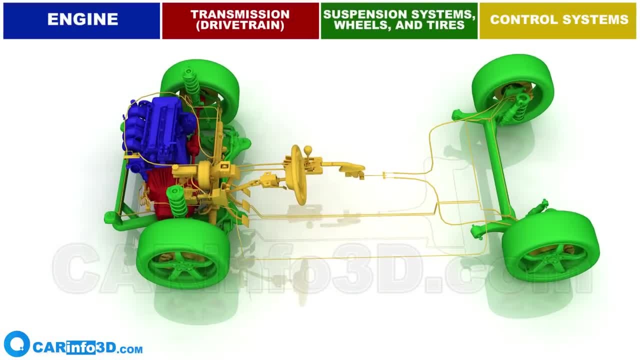 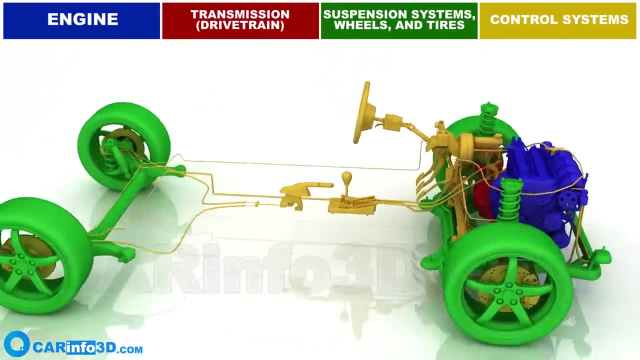 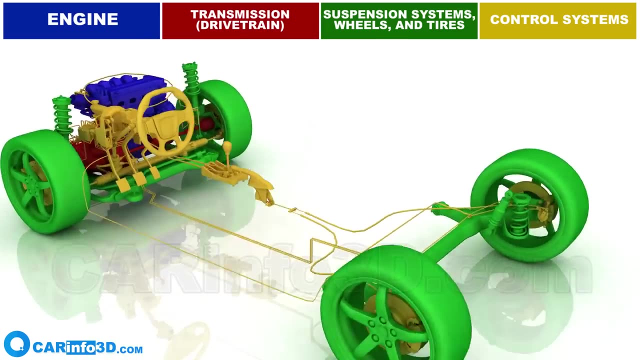 Let's take a look at the car's major components and assemblies. It may appear complicated now, but we're going to explore each system in greater detail. So let's look at car assemblies. We'll begin with the body and frame. This is the body. 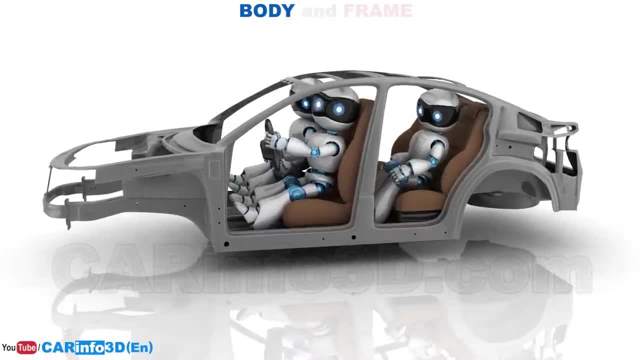 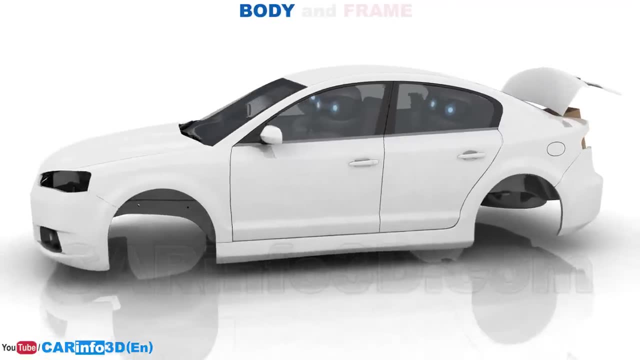 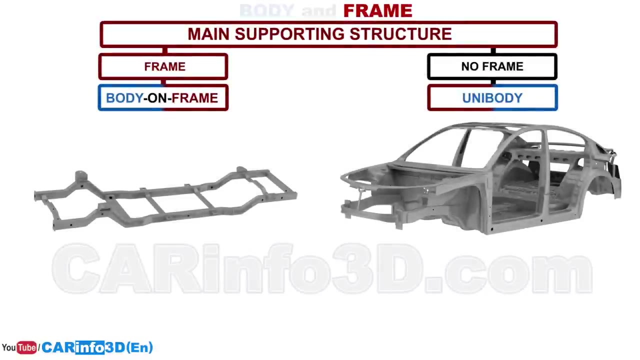 It provides space for the driver, passengers and cargo. This is the body, together with all auxiliaries and decorative elements. Next comes the frame. It is the main supporting structure to which all other components are attached. It can be a body on frame or a unibody construction. 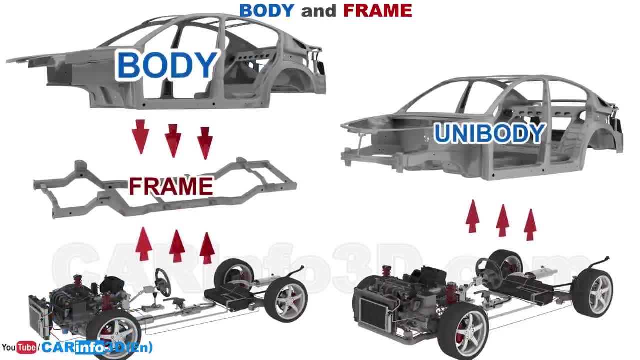 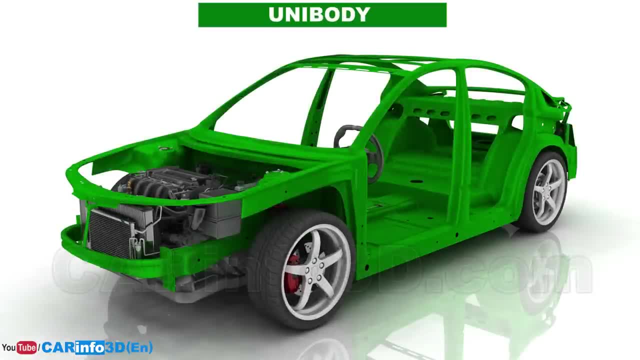 The unibody combines the function of the body and the frame. Most modern cars use this type of construction. Body on frame vehicles are much rarer and primarily comprise off-road SUVs. The next vehicle system is the engine. The engine is usually located in the front of the vehicle. 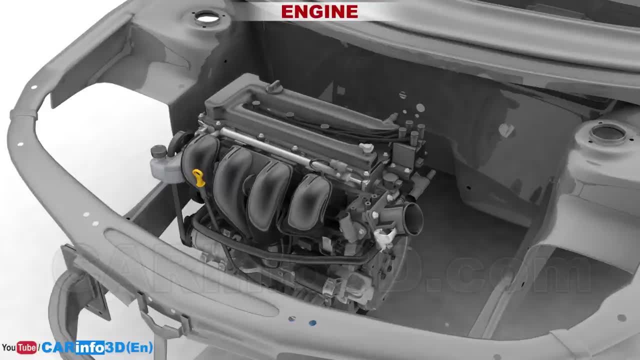 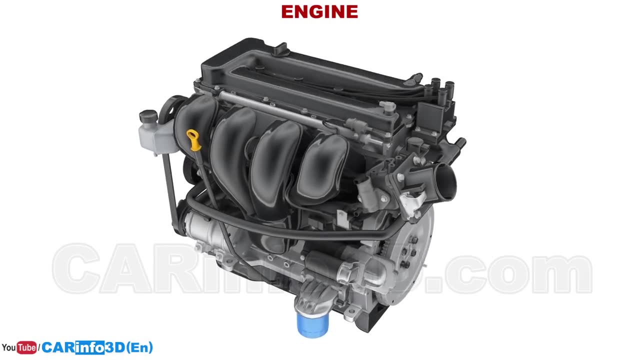 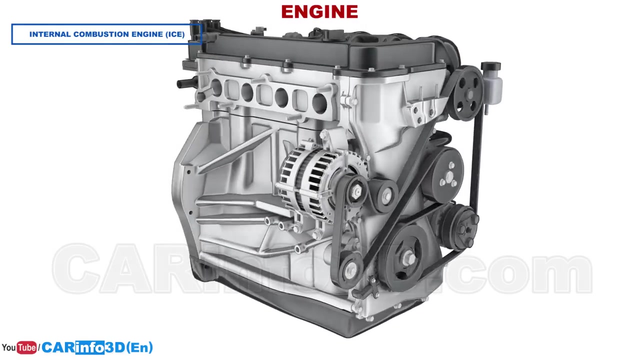 The engine converts one form of energy into mechanical energy, which is then used to propel the car. The internal combustion engine- ICE- is the most commonly used engine type in automobiles. Such engines rely on the combustion energy of gasoline, diesel fuel or, in rare cases, in the car. 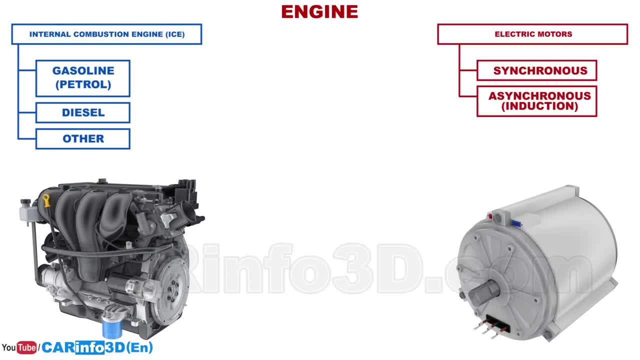 This engine is in fact used in the history of Mercedes-Benz, Panda, Porsche, Audi, Porsche and Opel, and so on. This favorite engine is often the only one not in the single-prime class. It is the most commonly used engine type in the amount of gas produced. 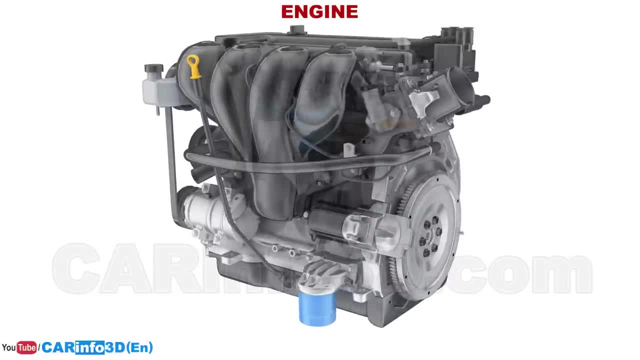 The engine is also Vienna engines, but not as many as those of Audi and Nissan. In this way, the engine is not a regular diesel engine. The engine is a multi-primed diesel option. The engine of the Mercedes-Benz is a 4-cylinder, V4-to-4-cylinder, V4-to-4-cylinder. 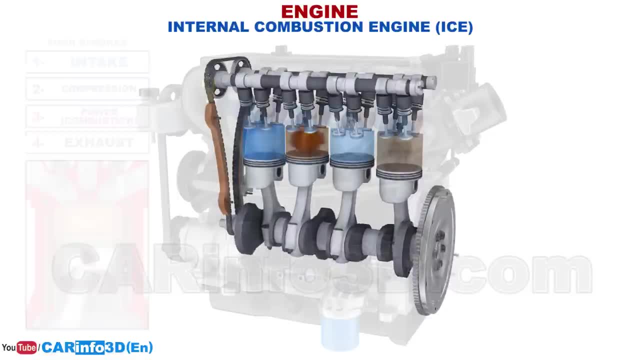 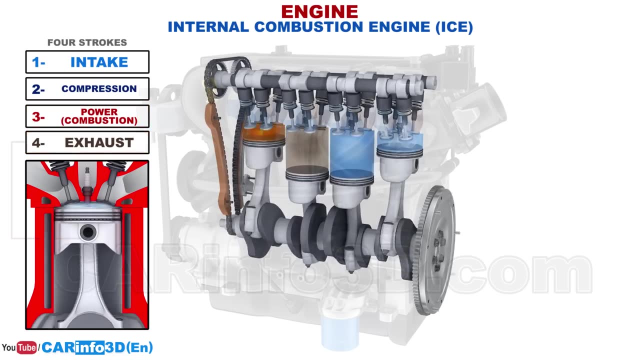 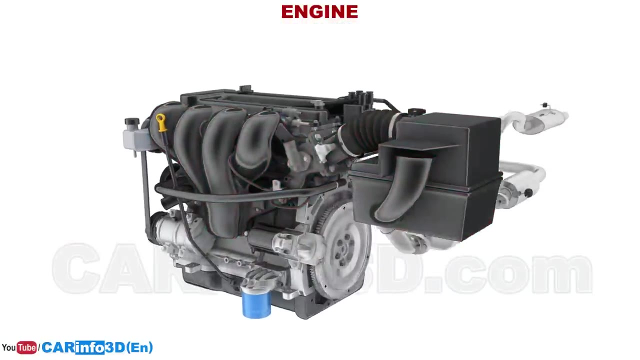 2.0-liter gasoline fuelressed engine. 2.0-liter diesel fuel-rich engine. 1.0-liter diesel fuel-rich engine. 2.0-liter diesel fuel-rich engine. 1.0-liter diesel fuel-rich engine. The engine has numerous subsystems, such as the intake system. 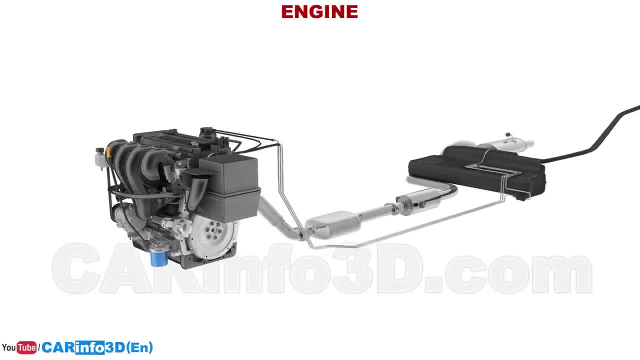 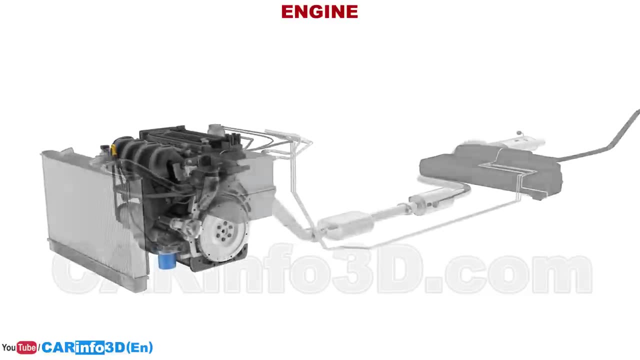 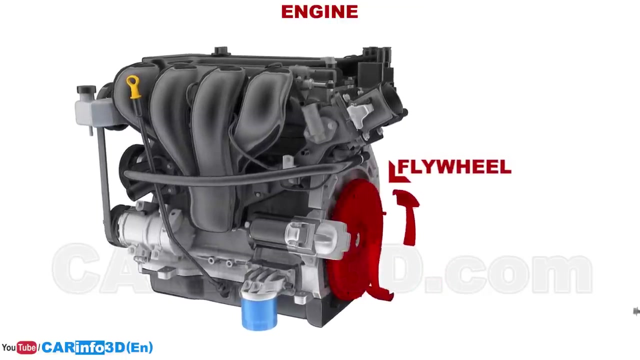 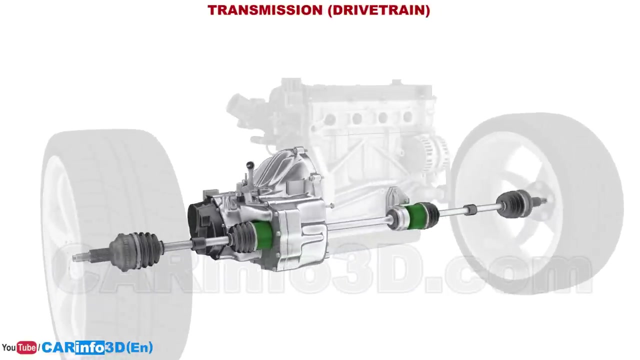 exhaust system, fuel supply system, cooling system and others. The internal combustion engine generates mechanical work and the torque is then transferred to the transmission system via a flywheel. The transmission is the device that connects the engine to the drive wheels. It transfers changes and distributes torque to the drive wheels. 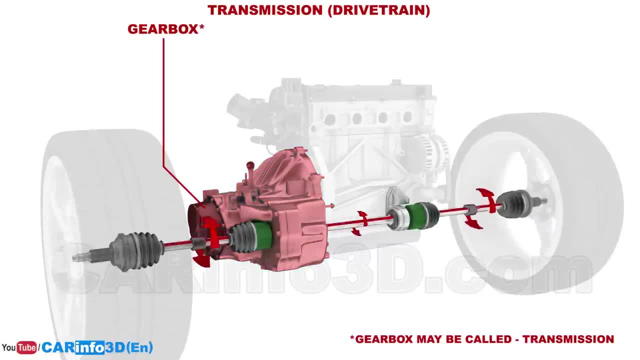 Transmissions are classified based on the type of gearbox. The manual gearbox requires the driver to select and change gears by using a gear shift lever and a clutch pedal. In case of the automatic gearbox, the driver only needs to shift the selector into the drive mode. 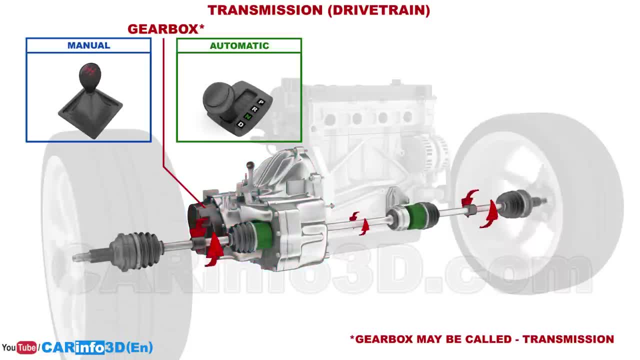 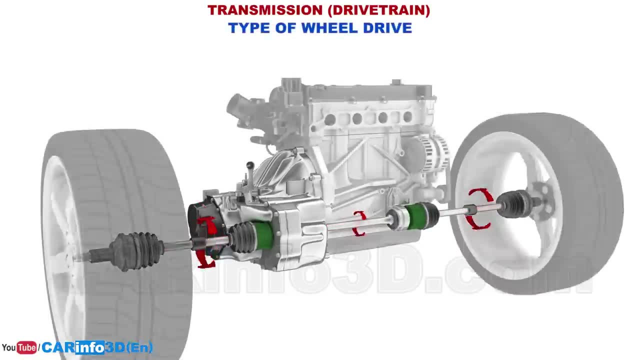 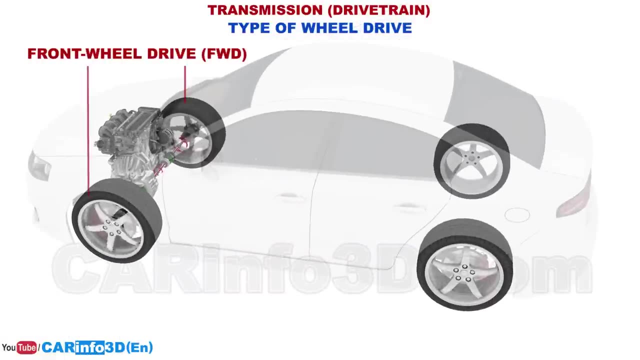 Further gear changes do not necessitate driver intervention. The type of wheel drive is another significant distinction between transmission systems. You can now see a vehicle with front wheel drive. Depending on the type of wheel drive, transmissions can have a variety of structures and compositions. 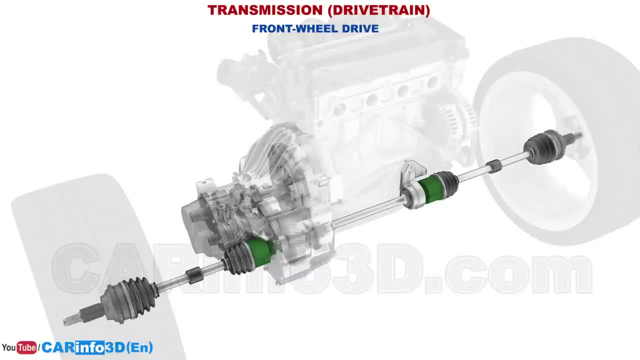 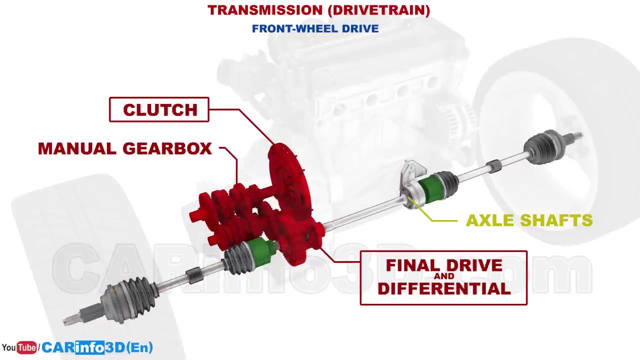 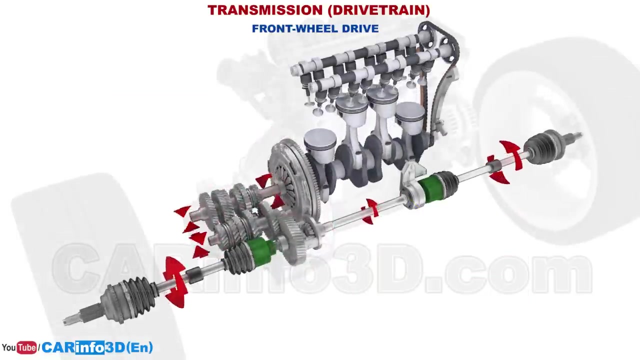 A front wheel drive. manual transmission includes the following components: The clutch, manual, gearbox, final drive and differential and axle shafts. The clutch, final drive and differential are all contained within the same housing as the gearbox. Now we can see how the engine and the transmission interact. 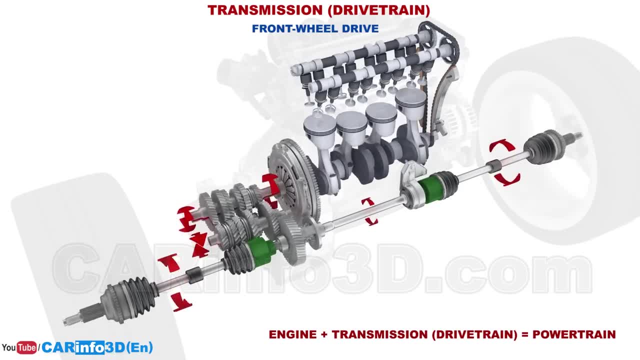 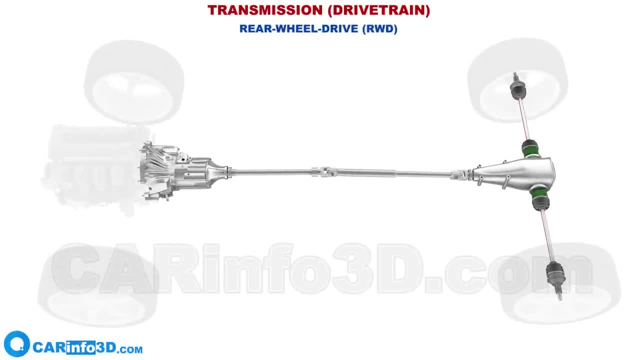 The combination of the engine and the transmission system is called the powertrain. Rear wheel drive is another type of wheel drive. Such transmission also include a propeller shaft. The final drive and differential are located on the drive axle outside the gearbox housing. 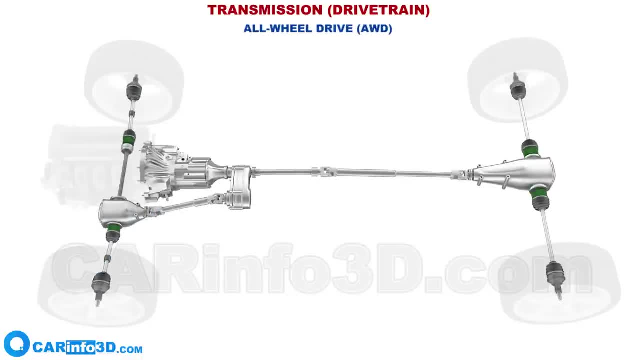 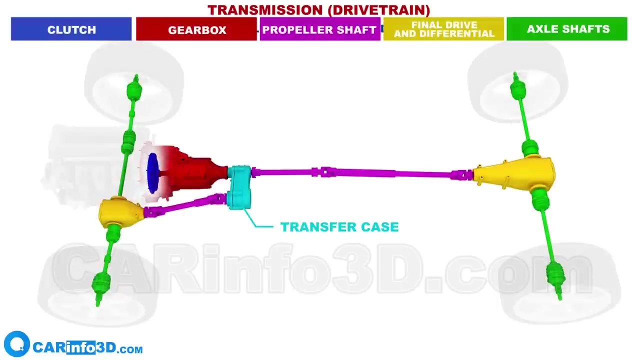 And this is an all-wheel drive transmission. In this case, torque is supplied to both axles full time or on demand. Its components also include a transfer case which can be installed in the same housing as the gearbox, The differential final drive and propeller shaft. 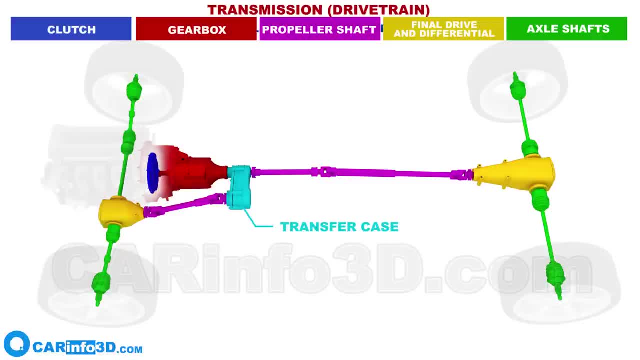 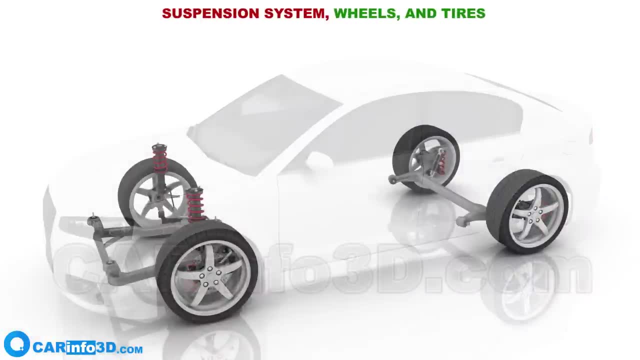 are duplicated on the driving axles, Let's return to the front wheel drive transmission and move on to the next systems: The suspension system. wheels and tires help a vehicle move along a road and receive and absorb the impact from various bumps, making driving safer and more comfortable. 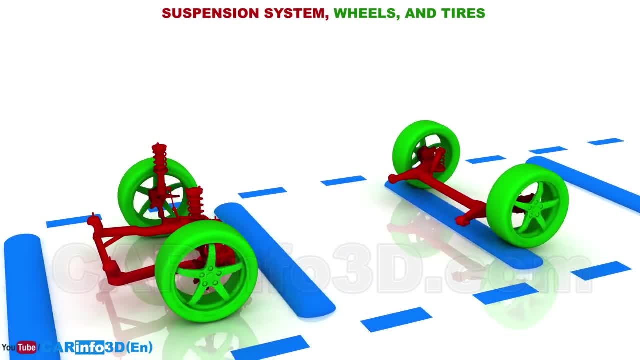 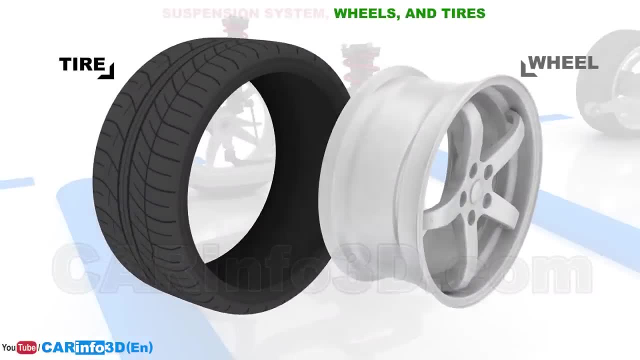 First, let's take a quick look at the wheels and tires. Wheels can be made from a variety of materials and in a variety of styles. They are surrounded by tires, creating an air-filled chamber. Sometimes, tires are also equipped with an inner tube. 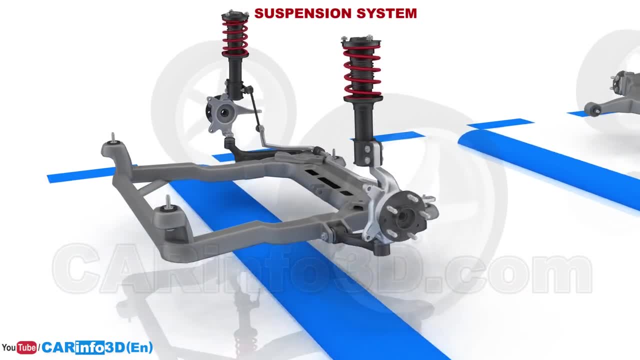 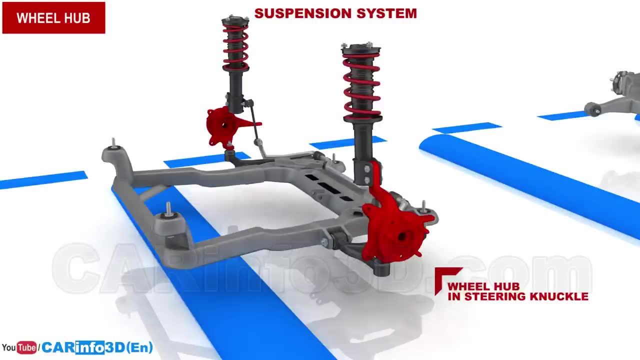 Let's go back to the suspension system. The suspension includes the wheel hub. This is a wheel hub mounted on a steering knuckle. The spring- a coil spring in our case- Shock absorbers, Suspension links, arms and beams. This type of suspension has an arm control. 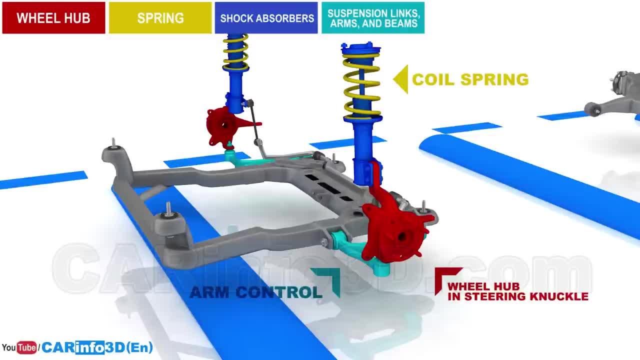 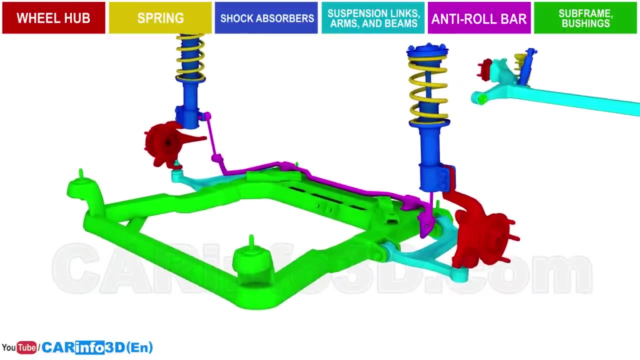 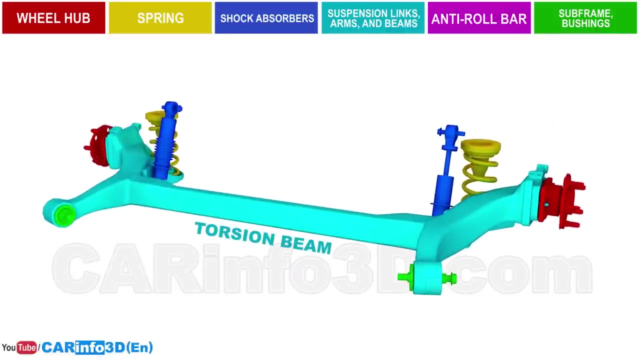 and a shock absorber that performs an additional function of the suspension arm, The anti-roll bar, The subframe and bushings. The front bar of the suspension system uses MacPherson struts, which are very popular among car manufacturers. On the rear axle we can see a semi-independent suspension. 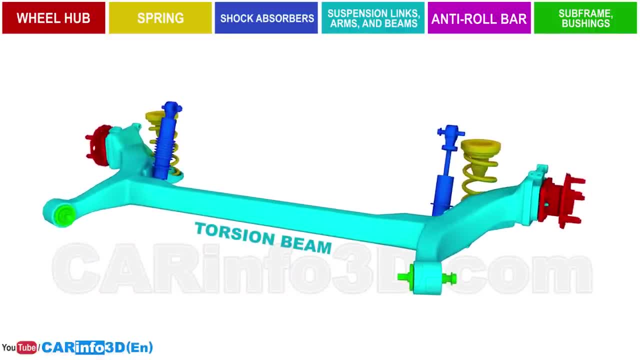 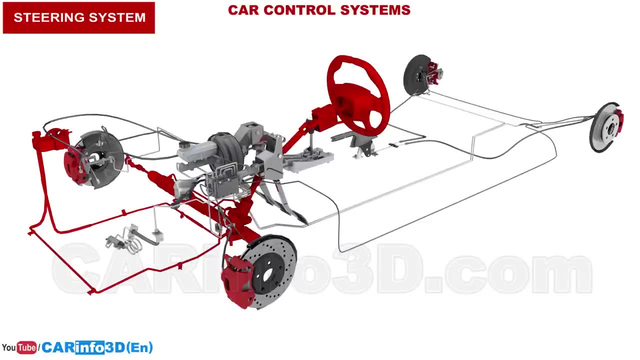 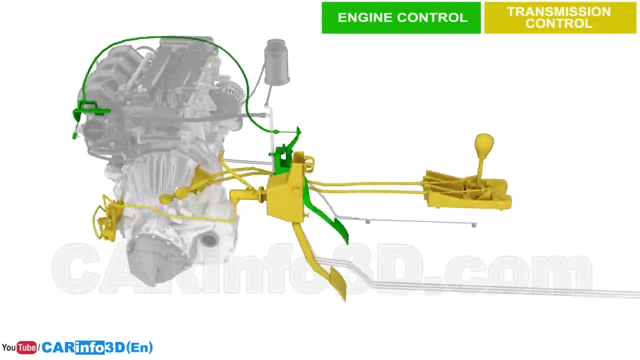 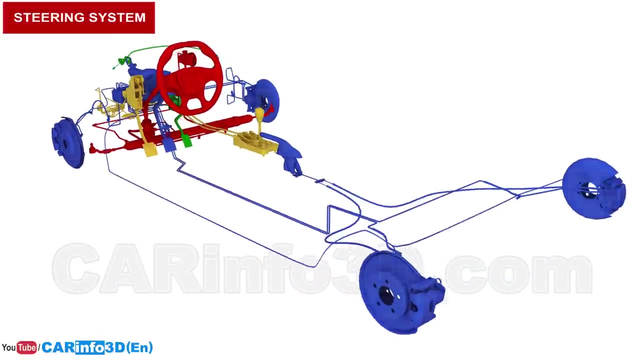 with a torsion bar. Next, car control systems. They include the steering system, the braking system. In this section it would also be appropriate to review engine and transmission controls. The steering system is required to change the direction of the car's movement. 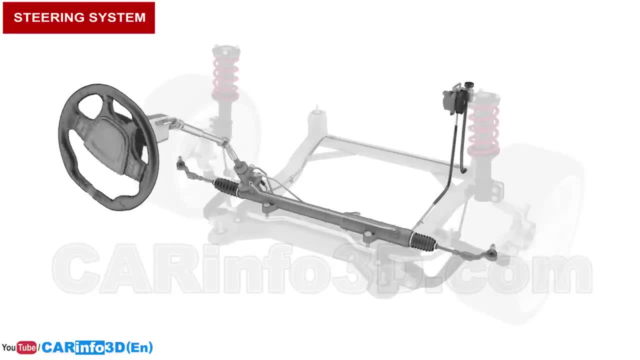 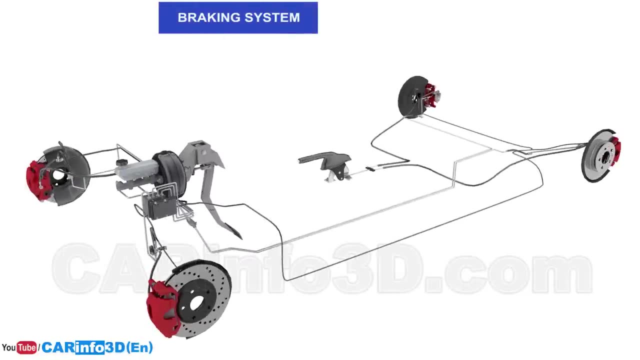 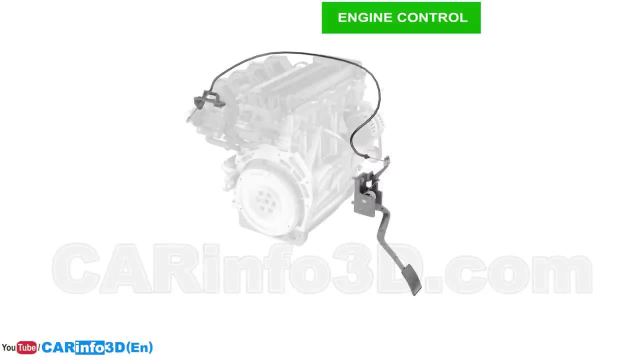 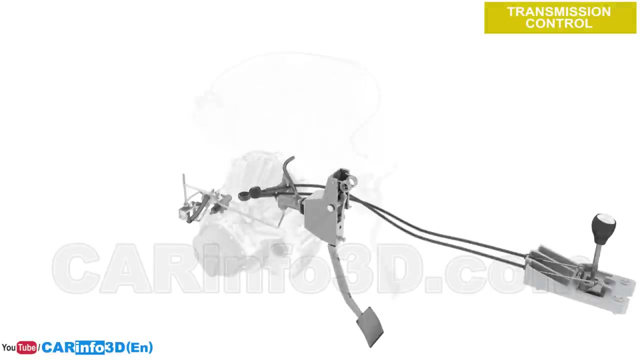 The braking system is required to slow down and stop the car, as well as to keep it in place. Engine control is used to alter the engine torque. This is an obsolete model with a mechanical throttle valve. Transmission control is required to temporarily disconnect the engine and the transmission.